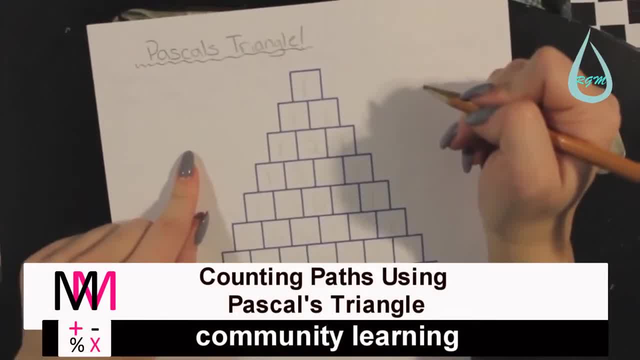 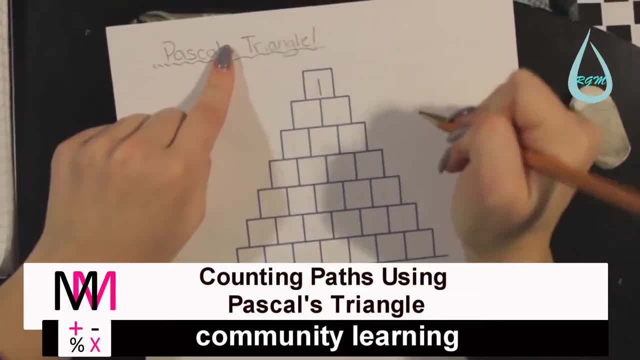 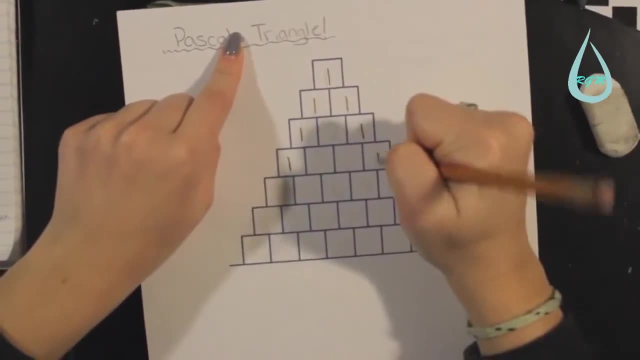 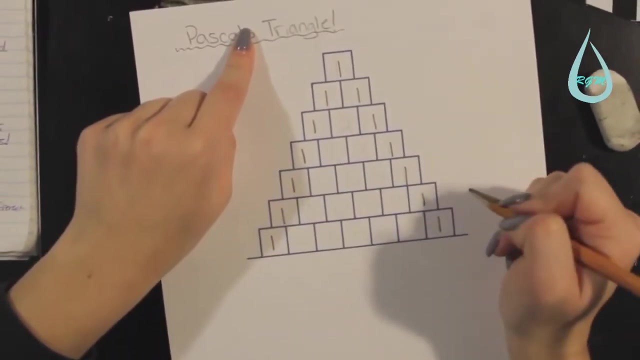 Pascal's Triangle is a number pattern named after Blaise Pascal, a famous mathematician and philosopher. Pascal's Triangle begins with a 1. at the top of the triangle, Each row begins with a 1 and ends with a 1.. In order to continue Pascal's Triangle, add the. 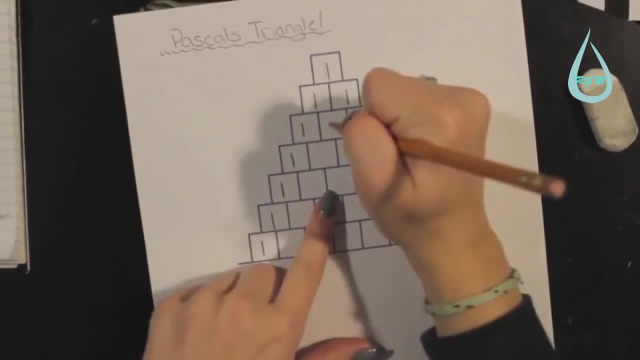 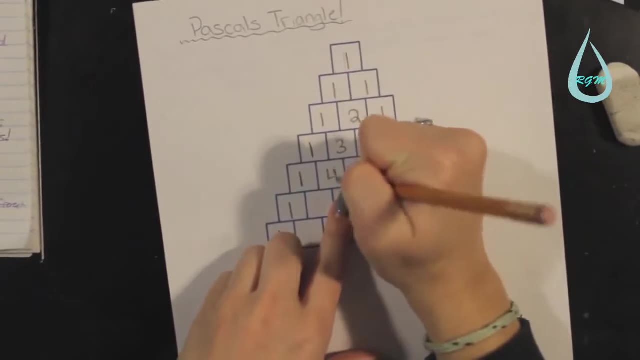 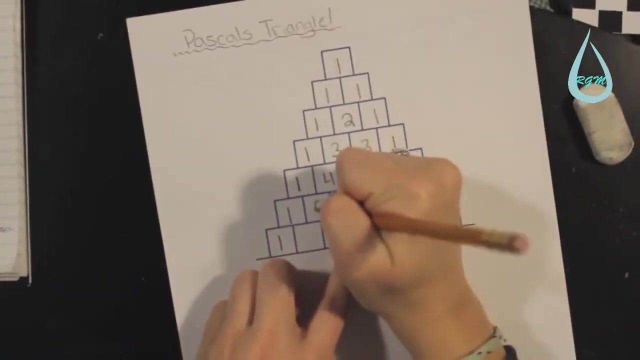 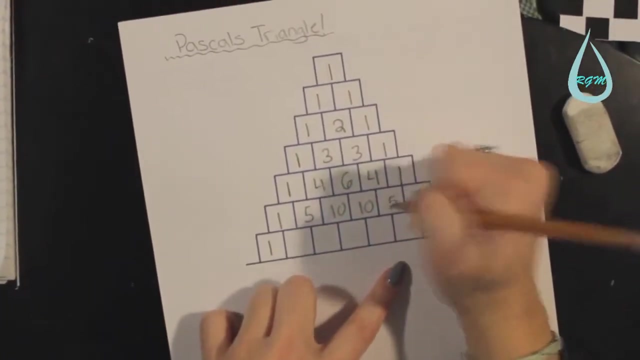 two numbers directly above it together, So 1 and 1,, 2. 1 and 2,, 3.. 2 and 1,, 3.. 1 and 3,, 4.. 3 and 3,, 6.. 3 and 1,, 4.. 1 and 4,, 5., 4 and 6,, 10.. 6 and 4,, 10.. 4 and 1,, 5.. And you, 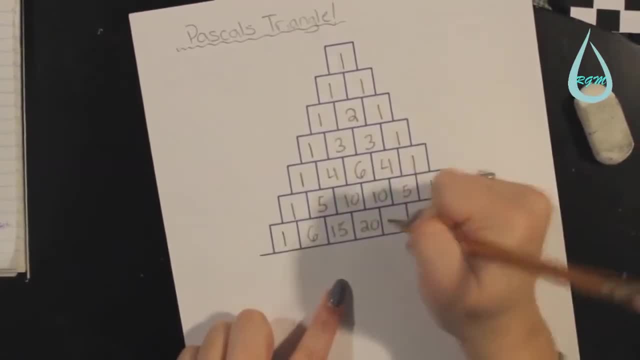 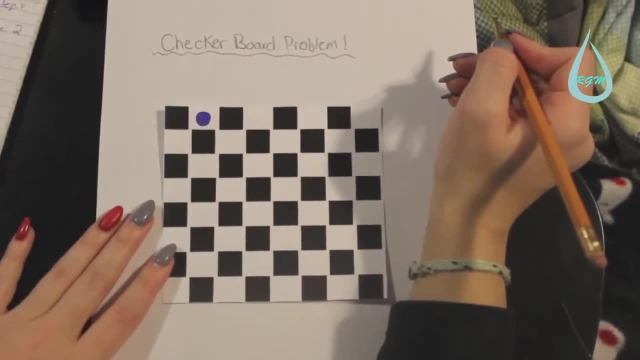 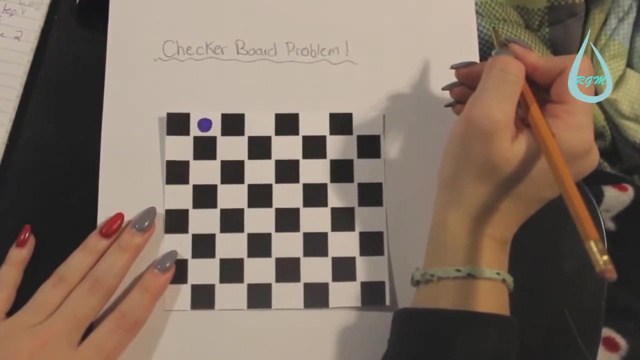 just continue until the very bottom. Pascal's Triangle can be used to determine the probability of many different pathways to a certain destination. An example of this could be a checkerboard. Count the number of paths for the checker to reach the bottom of the board. So this would be the beginning. 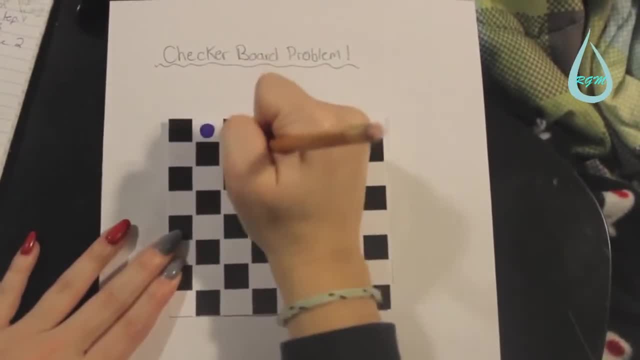 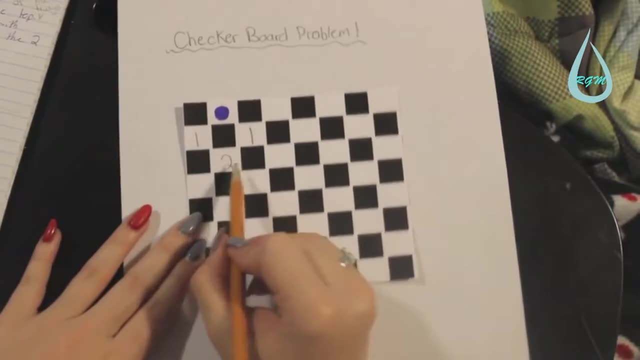 of Pascal's Triangle. So this would be 1,, 1, 1.. And again you're going to add the two above numbers together. As you can see, here we run into a problem Because there isn't a number to add over here, So we just have to continue on with. 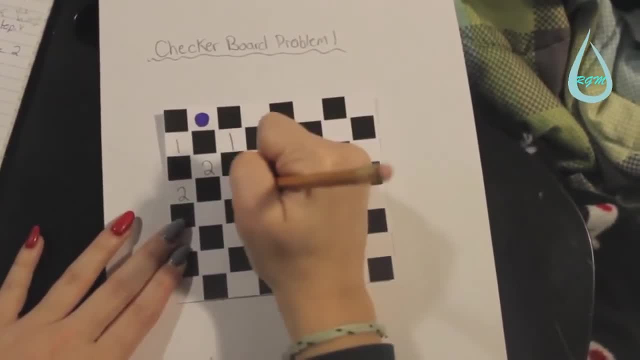 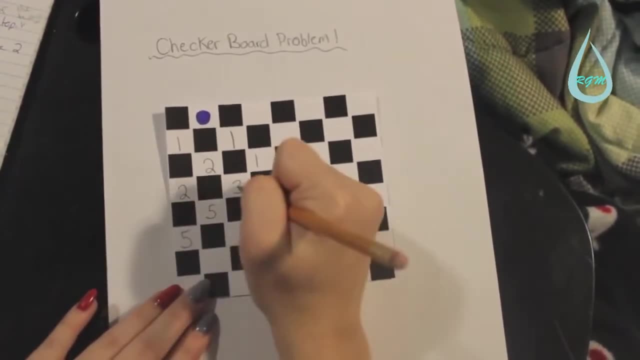 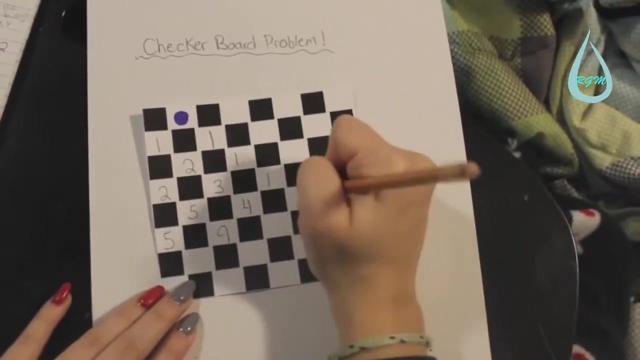 2.. This is a 1,, so this will be 3.. Add these together, 5.. Same problem: we continue: 5.. 1, 4.. Add these together: 9.. Again, there's 1s going all the way down the side 4 and 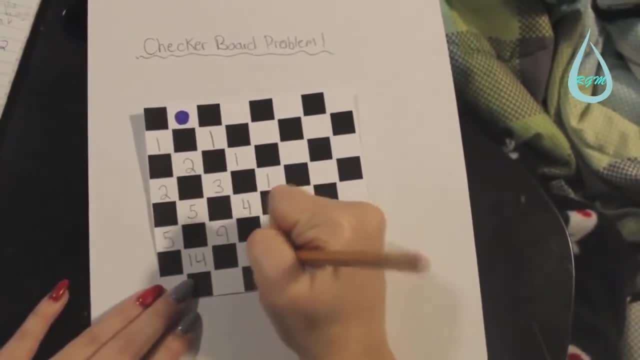 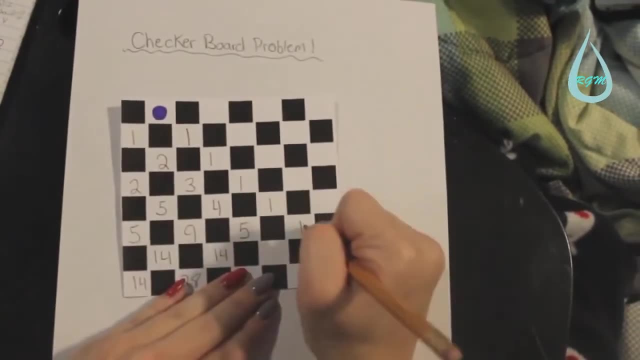 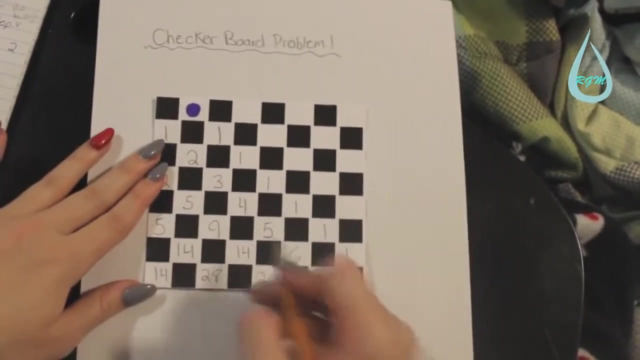 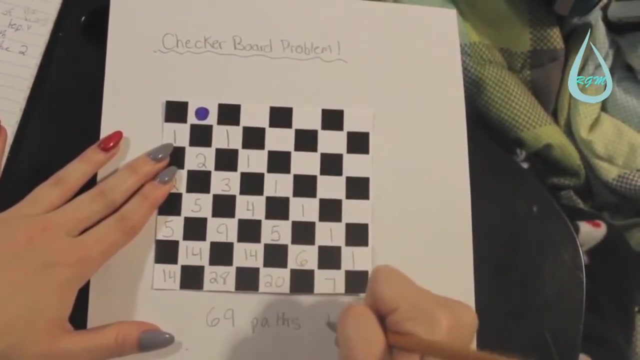 1 is 5.. 14.. 14. 14 continues this way, 28.. 5 and 1 is 6.. 20,, 7.. And then you're going to add all these totals together and it's going to be 69 paths to the bottom of the board.